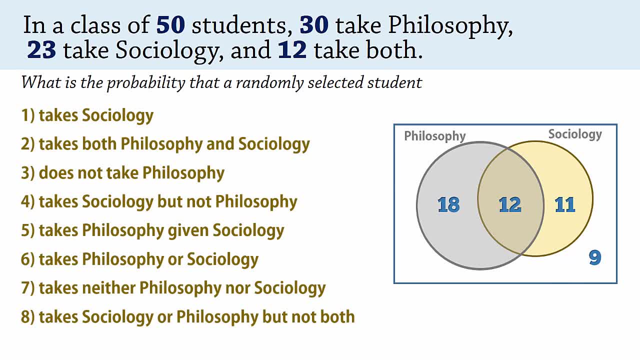 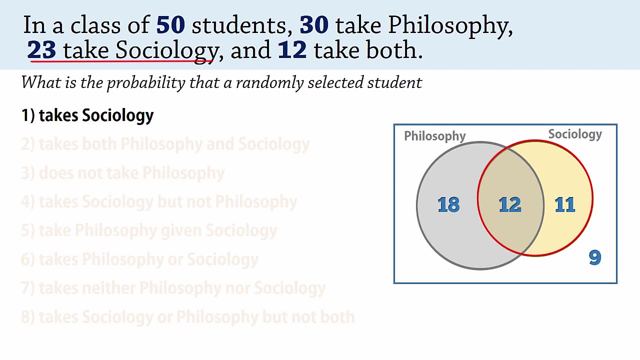 In essence, the four values must add up to 50. And we can convert them to probabilities if we want, but in a more simple way. But let's just leave them as numbers…. Number 1- Since 23 students take sociology, the probability that a student takes sociology is: 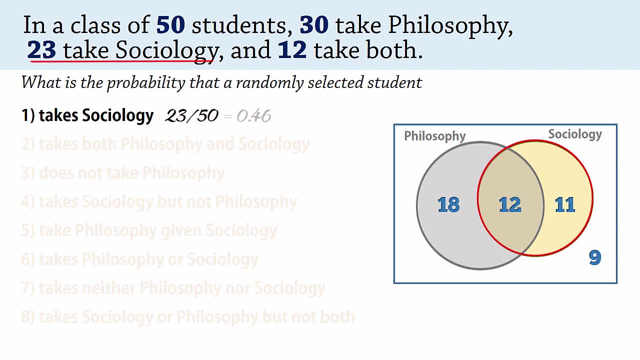 simply while forgetting that total take is 23 divided by 50,, which is Logical Component Number 2-. The probability of a student taking philosophy AND sociology is the joint probability represented by this intersection, whether a student takes philosophy or sociology, which is 22 times 50,, which is red fact, and 23 divided by 52,, which is 20ans expressions. Well, I am going to leave them as numbers. Number 2- Since 23 students taken sociology, the probability that a student takes sociology is simply 23 divided by 50, which is 0.46.. Number 2- The probability that a student taking philosophy or sociology. 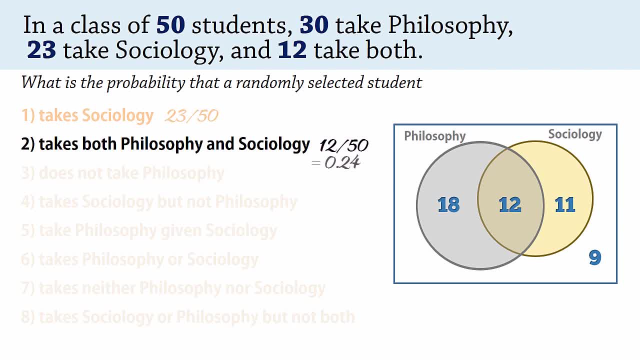 For number 3,, the probability that a student does not take philosophy can be found using the complement rule, that is 1 minus the probability that a student takes philosophy, which gives 1 minus 30 over 50, and that gives 20 over 50, or 0.4.. 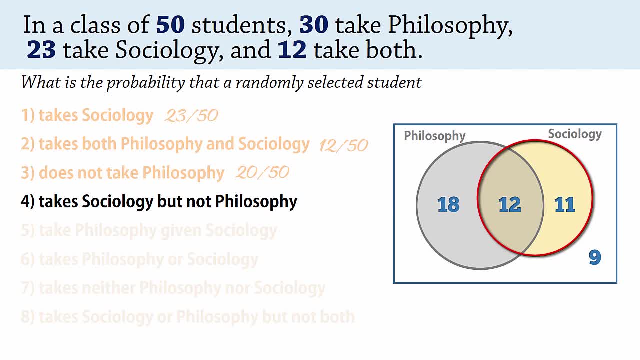 For number 4, note that of these 23 students that take sociology, 12 of them also take philosophy, So the remaining 11 here take sociology but not philosophy. that is sociology only. Therefore, the probability is 11 over 50, which is 0.22.. 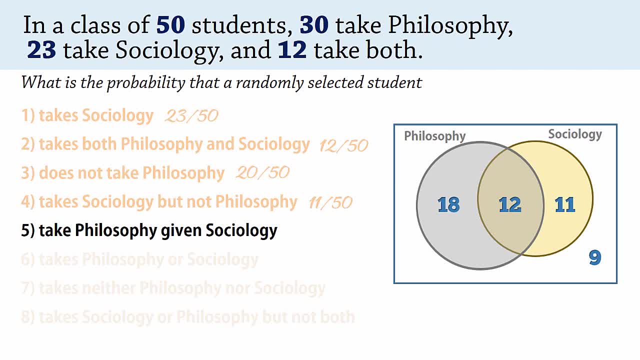 In number 5, we want the probability that a student takes philosophy, given that the students take sociology. This is basically asking: out of the students taking sociology that is given sociology, what proportion also takes philosophy, Since out of the 23 students taking sociology, 12 are also taking philosophy. 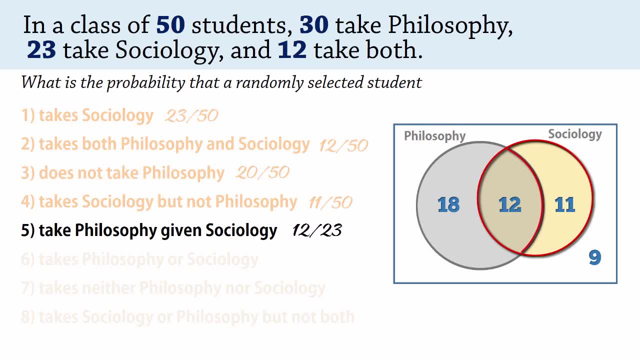 The probability is therefore 12 divided by 23,, or 0.52.. For number 6, philosophy or sociology means the union of these two. So we want the probability that a student does not take philosophy. So we want the probability that a student does not take philosophy. 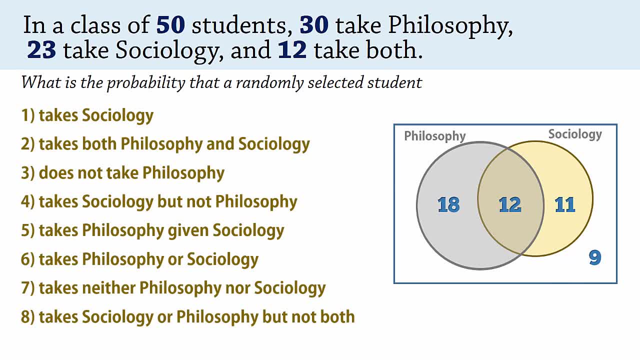 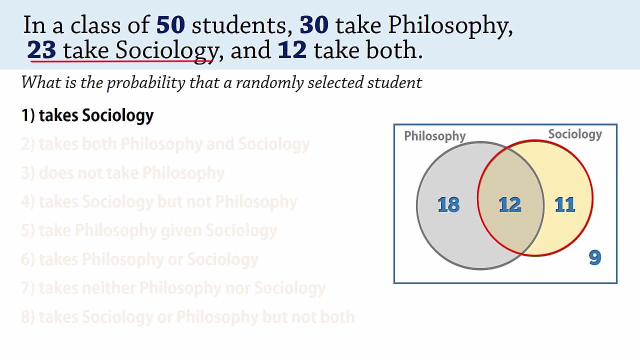 In essence, the four values must add up to 50. And we can convert them to probabilities if we want, or to percent, But I'm just going to leave them as numbers Number one, since 23 students take sociology. the probability that a student takes sociology is simply 23 divided by 50, which is 0.46. 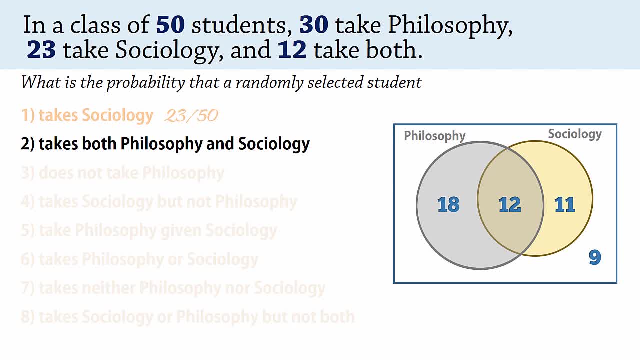 Number two, the probability of a student taking philosophy and sociology is the joint probability represented by this intersection, which is 12 divided by 50, or 0.24.. For number three, the probability that a student does not take philosophy can be found: 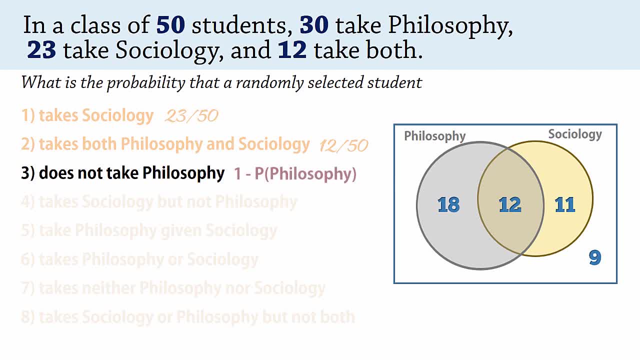 using the complement rule, That is 1 minus the probability that a student takes philosophy, which gives 1 minus 30 over 50, and that gives 20 over 50 or 0.4.. For number four, note that of these 23 students that take sociology, 12 of them also take philosophy. 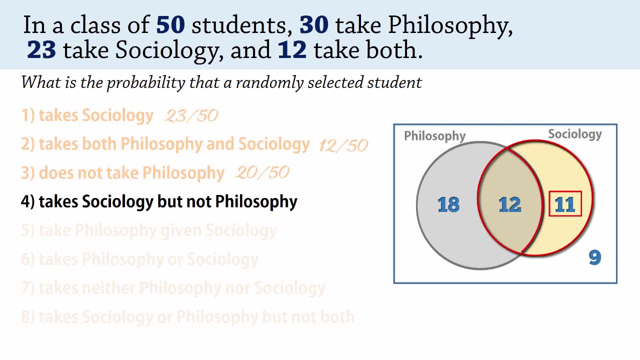 So the remaining 11 here take sociology but not philosophy. That is sociology only. Therefore, the probability is 11 over 50, which is 0.22.. In number five, we want the probability that a student takes philosophy, given that the students take sociology. 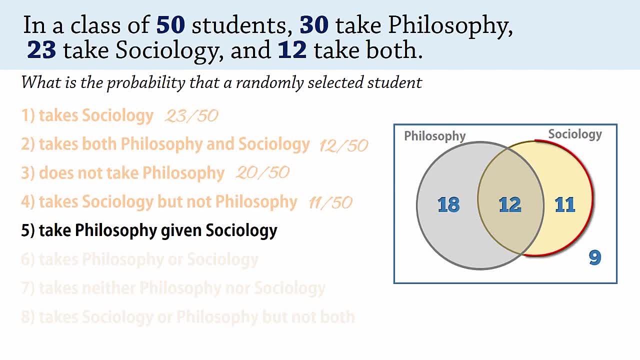 This is basically asking: out of the students taking sociology that is given sociology, what proportion also takes philosophy, Since out of the 23 students taking sociology, 12 are also taking philosophy. The probability is therefore 12 divided by 23 or 0.52.. 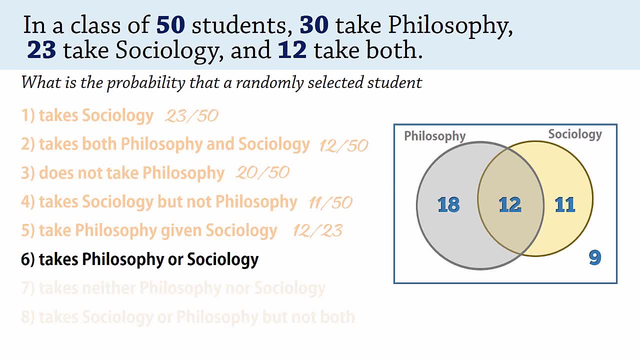 For number six, philosophy or sociology means the union of the two events, And that represents students that take philosophy or sociology, or both. We can then use the addition rule or simply add these three values and then divide by 50.. Adding the three values gives 41.. So the probability is 41 divided by 50, given 0.82..